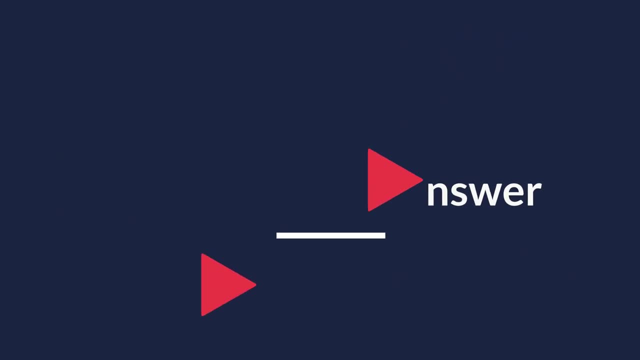 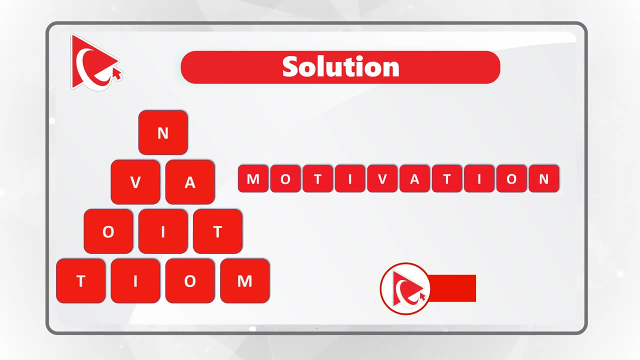 The word motivation, for example, is M O T I V A T I O N, And motivation defaults on why a person acts in a particular way. How does everyone behave or behave? This is somewhat obvious. As you can see, it's rather detailed. 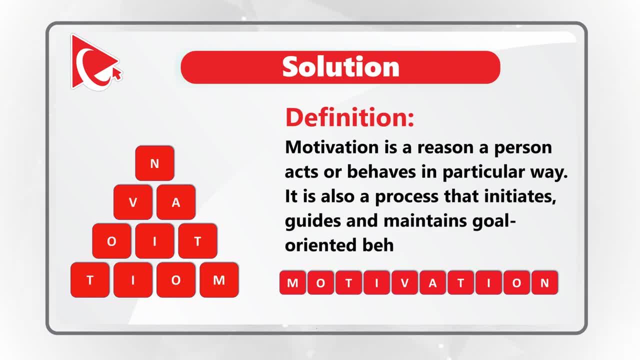 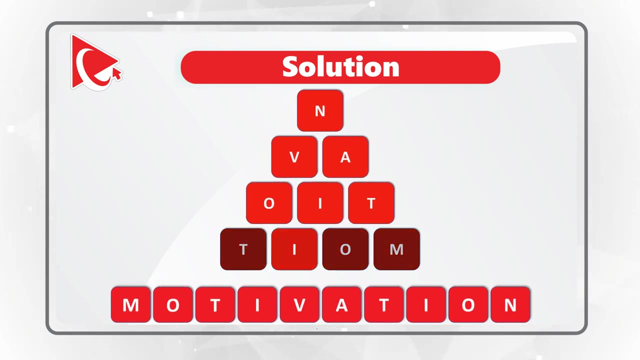 in particular way. it is also a process that initiates, guides and maintains goal-oriented behaviors. believe it or not, but doing more practice exercises helps you get better with the skill of forming the word. for example, if you start with the bottom right corner, you can form the word motivation. you see m? o and then you swap t? i and then, if you continue, you go. 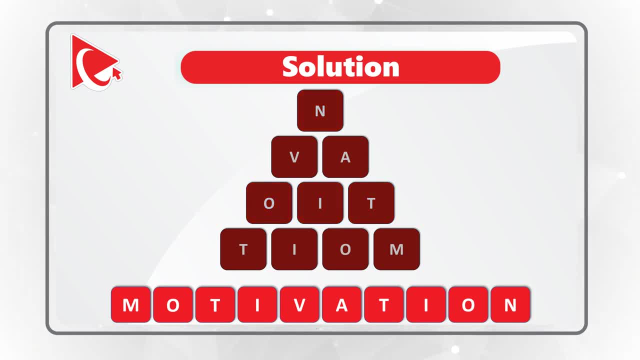 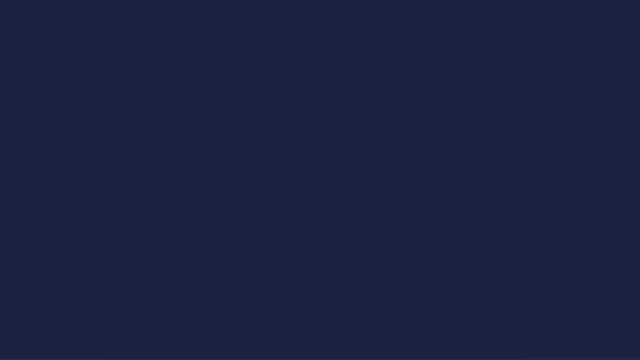 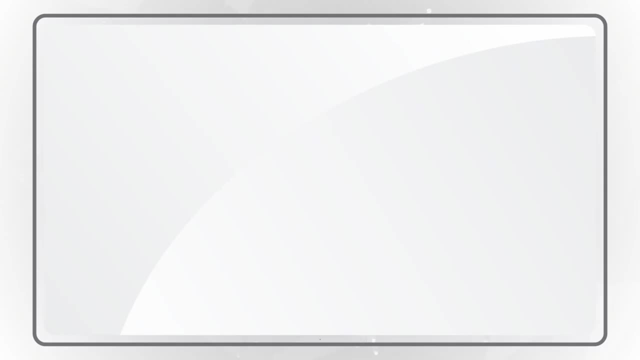 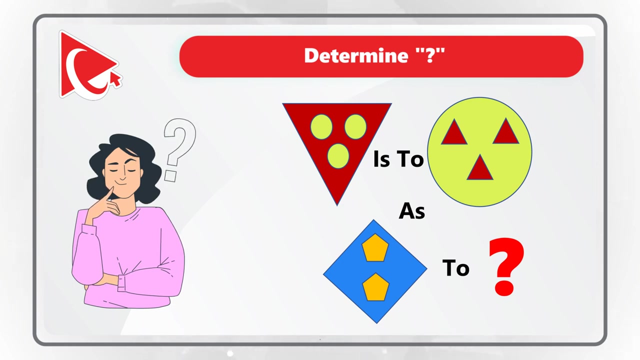 v a t i o n. you can solve these types of challenges better if you do more crosswords and puzzles. i love this question because you need to determine relationship between the shapes and you need to determine which shape has similar relationship to rectangle. if you take a close look, you will see that there are other smaller shapes. 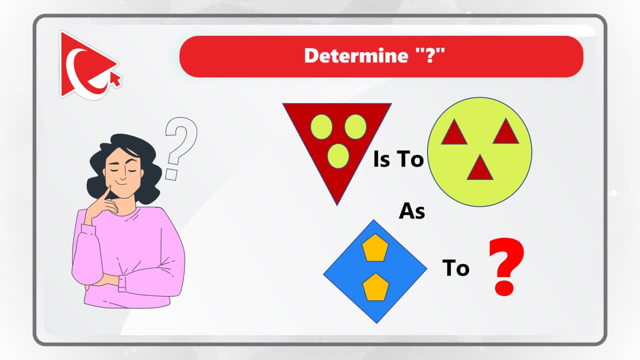 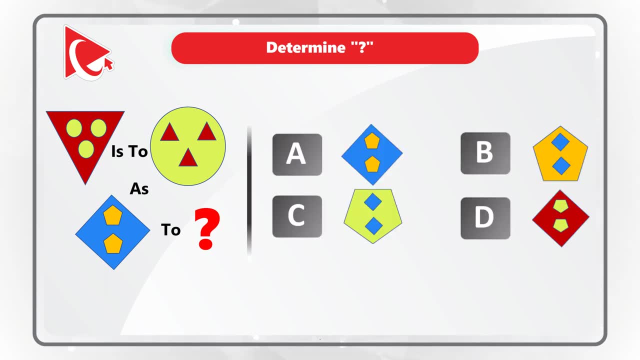 inside the larger shapes and you have four different choices to choose from the final answer: choices a, b, c and d. take a close look to see if you can come up with the answer. have you tried solving it? were you successful, let's move forward so we can get to the correct solution together. 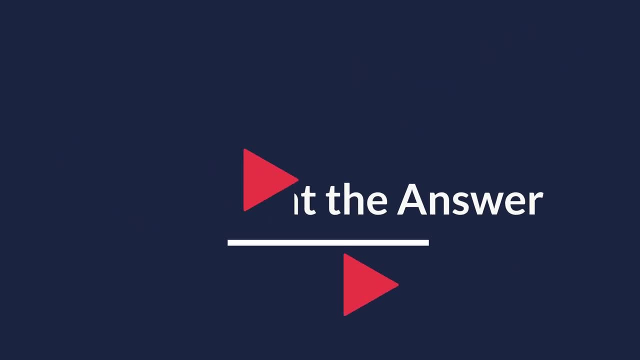 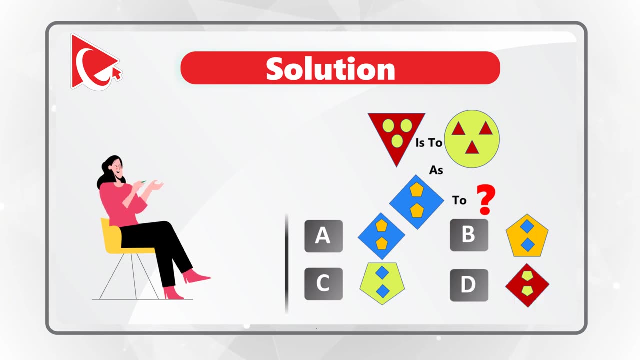 to determine the correct answer in this case and in a lot of other cases, you need to look for patterns, and the pattern in this particular case is that, to build the relationship, inside shape becomes outside shape, preserving the number of the inside to outside shapes ratio, if you look. 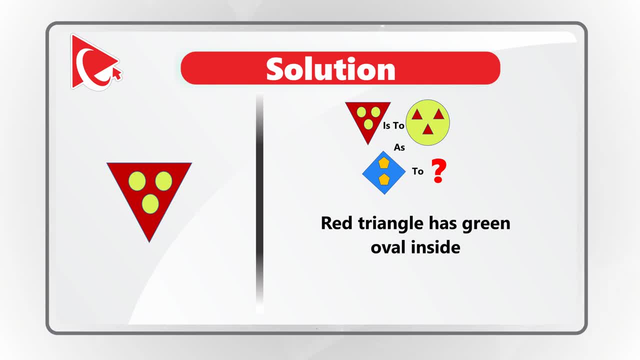 closely at the relationship presented in this question, you see that the red triangle has green ovals inside and it has a relationship to green oval that has red triangles inside. knowing this, we need to determine relationship of the blue square that has pentagons inside to one of four shapes presented in possible answers. do you see it now? all you need to do is take a close look. that question has pentagons inside to one of four shapes presented in possible answers. do you see it now? cause you see like a regular penguin. 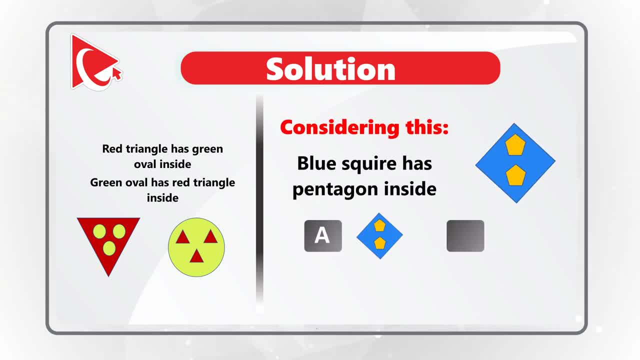 so a good means to connect with the resistance is not one of the primaryуг in interior need to do. in this particular answer is to take the pentagon, which is inside the square, enlarge it and put blue squares inside. So, as you might have guessed, the correct answer here is choice B. 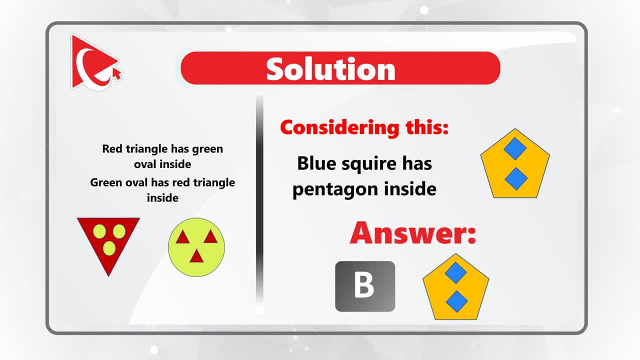 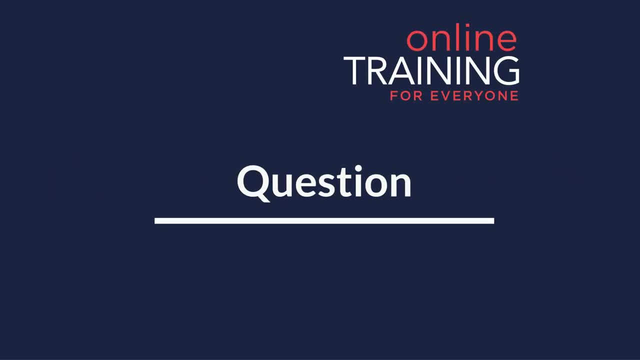 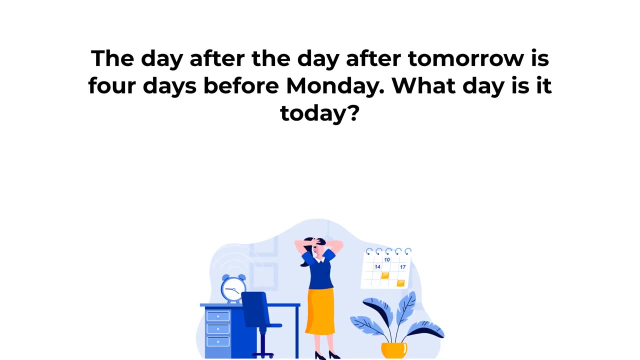 Hopefully you've nailed this question on your own and now know how to answer similar problems on the test. Here's the practice problem for you: The day after, the day after tomorrow is four days before Monday. What day is it today? You have four different choices: Choice A- Sunday. Choice B- Monday. 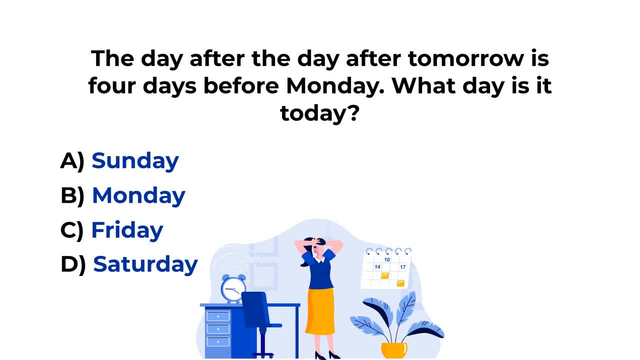 Choice C- Friday. Choice D- Saturday. Feel free to pause this video to see if you can come up with the solution. I would like to give you a hint. The best way to solve these types of problems is using reverse calculations. So do you see the answer? Give yourself 10 to 15 seconds to see if you can. 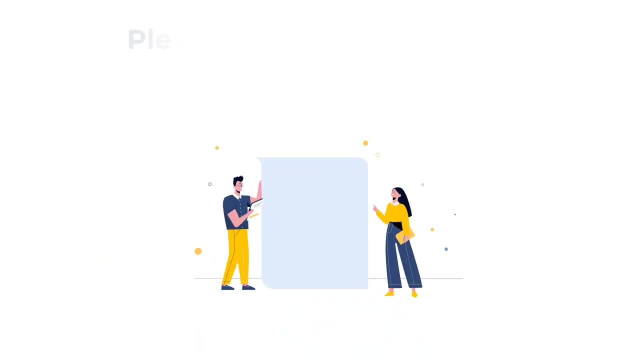 come up with the solution. Did you figure out the answer? Make sure to pause your answer, as well as your rationale for solving this problem, in the comment section of this video. Thanks for participating and good luck. Here is the frequent test problem. 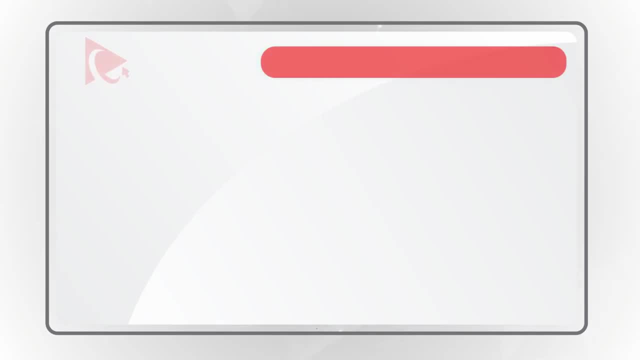 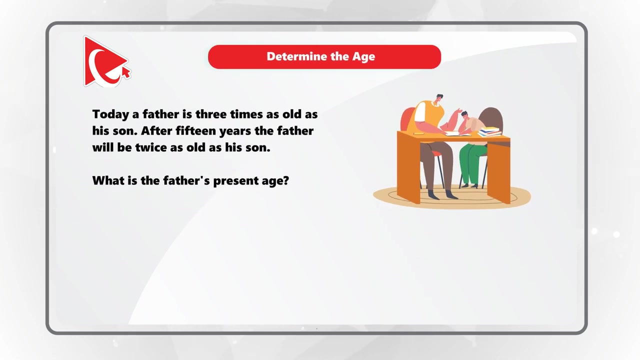 where you need to determine the age of the family members. Today, a father is three times as old as his son. After 15 years, the father will be twice as old as his son. What is the father's present age? And you have four different. 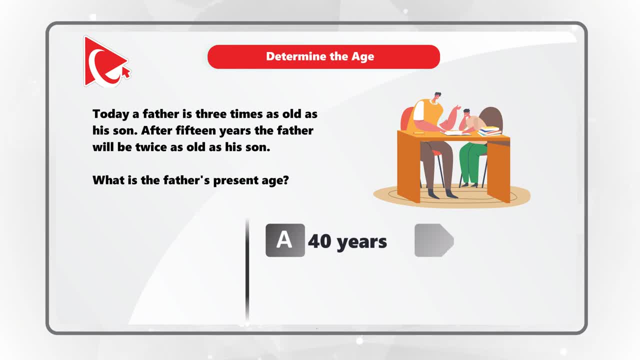 choices: Choice A- 40 years, Choice B- 45 years, Choice C- 50 years And choice D- 55 years. Do you see the answer? Give yourself a little bit of time to see if you can come up with the solution. 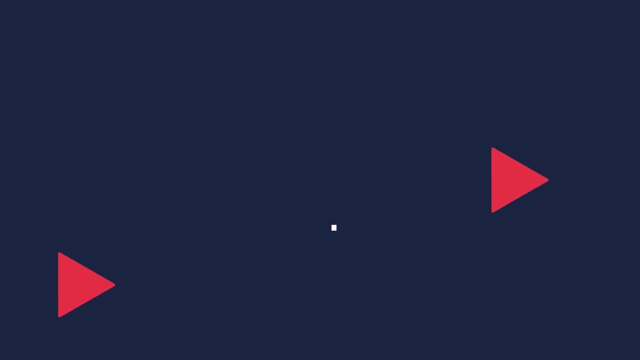 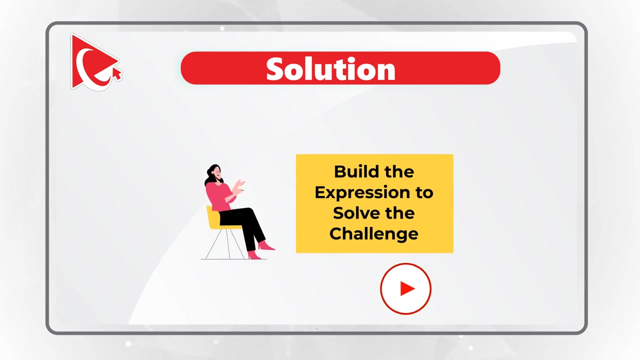 One of the ways to solve this problem is to take the number from the solution and see if it will work- the math. But instead of doing that, we're going to build the expression and calculate the father's present age. In the first step, we're going to introduce 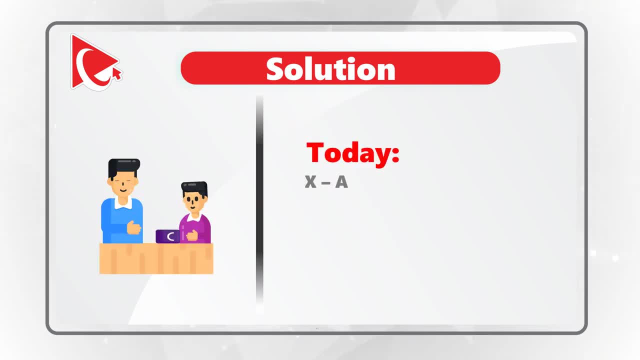 two variables. Variable X will represent age of the son today and variable Y will represent father's age today. So our first formula is: 3x equals Y, which indicates that today father is three times older than his son. After 15 years our expression will be different. 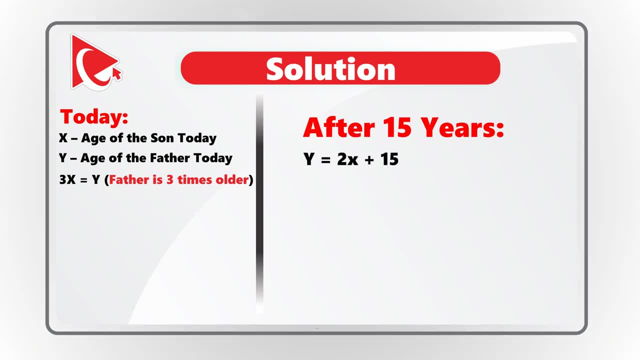 The new expression will be: Y equals Y, 2x plus 15.. Because in both cases y is the same, we can build a new expression: 3x equals 2x plus 15.. Once we simplify, 3x minus 2x will equal 15.. And after completing the calculations, 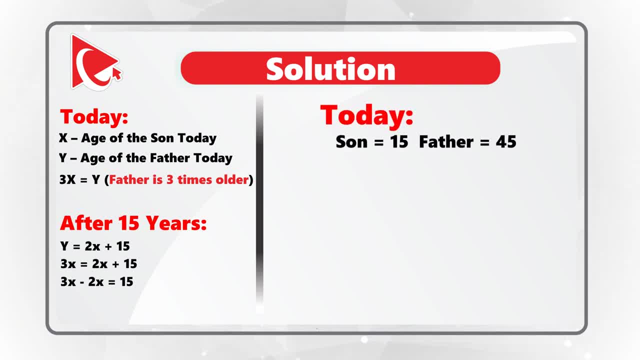 x will be equal 15 and y will be equal 45.. Based on this, today's age of the sun is 15 years old, which means that after 15 years, sun will be 30 years old and father will be 60 years old. 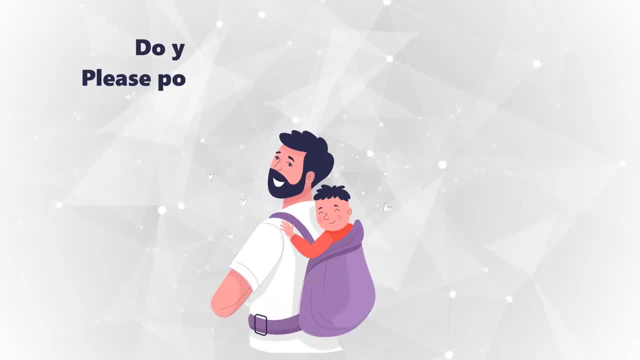 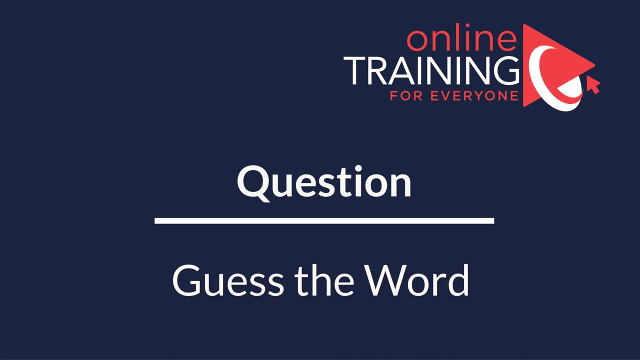 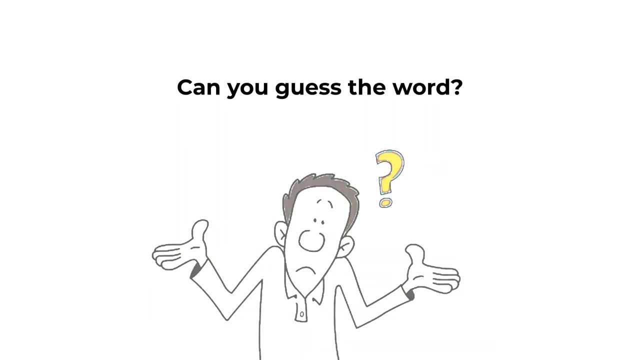 Hopefully you've nailed this question and now know how to answer similar age problems on the test. Here's the cool question that you frequently get on the test: You're presented with four different letters and you need to guess the word using all letters presented- The letters we have. 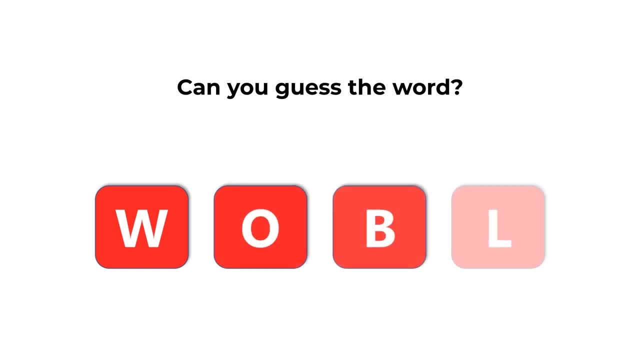 are W, O, B and L. Can you guess? Can you guess the word? Give yourself 10 to 15 seconds to see if you can come up with the answer. Ready or not, let's go ahead and reveal the solution. 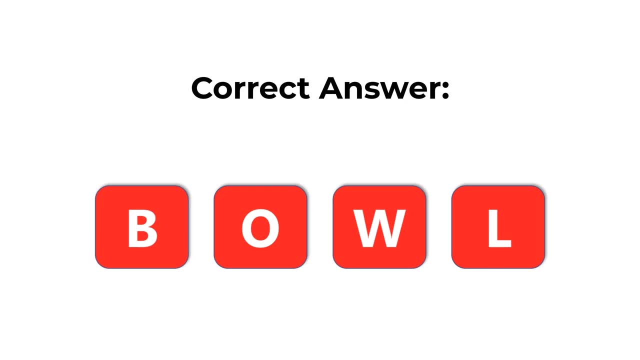 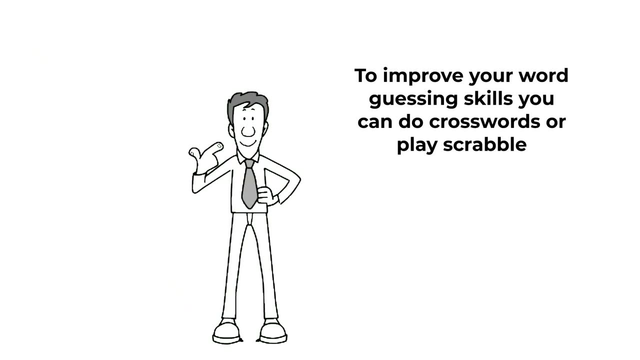 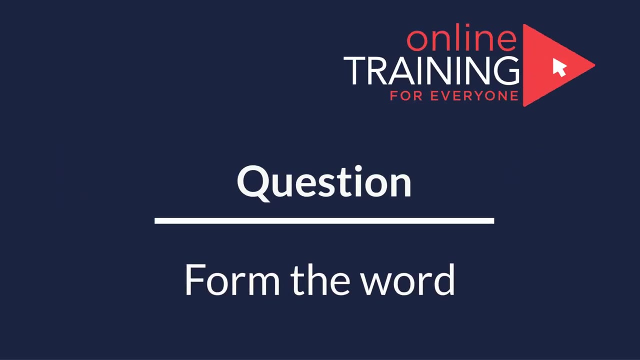 The correct answer here is BOWL, which is spelled as B-O-W-N-L. Hopefully you've nailed this question and now know how to answer similar problems on the test. Let's look at the interesting question where you need to form the word and you need to use all the 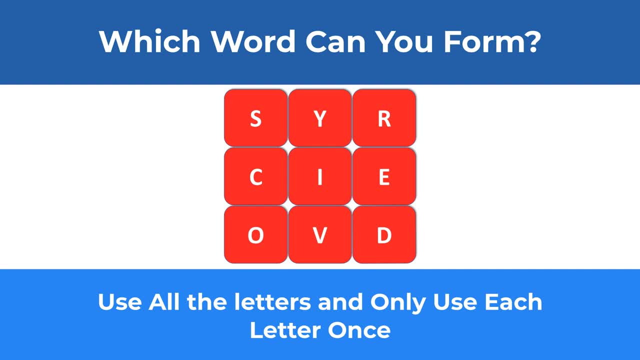 letters and only use each letter once You're presented with nine letters. Those nine letters are S, Y, R, C, I, E, O, V, D, and you need to form the word using all the letters. Do you see? 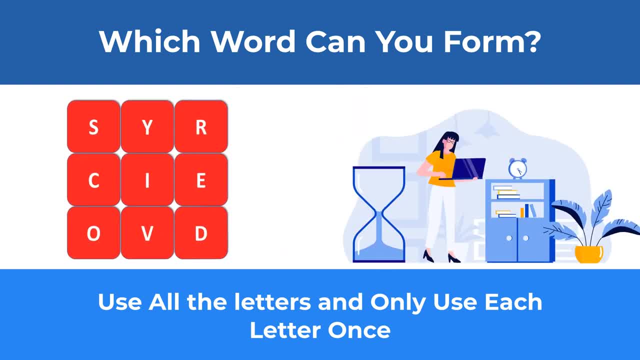 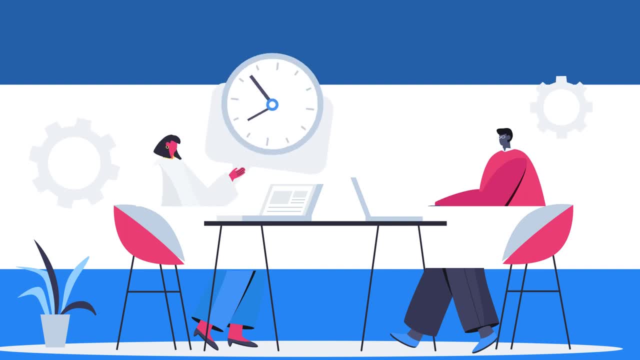 the solution. Give yourself a little bit of time, Maybe 10 to 20 seconds. This is typically as much time as you get in a real test, Ready or not. I am going to reveal you my version of the solution, But my version may not be the only one. 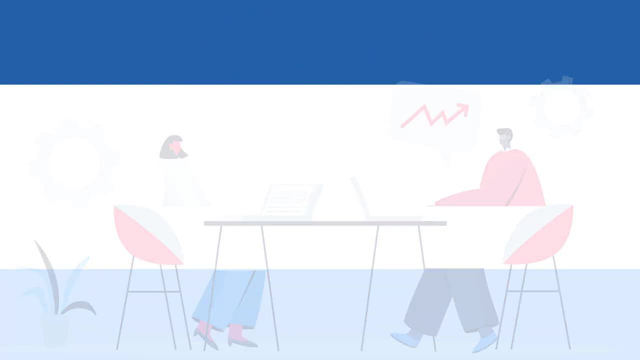 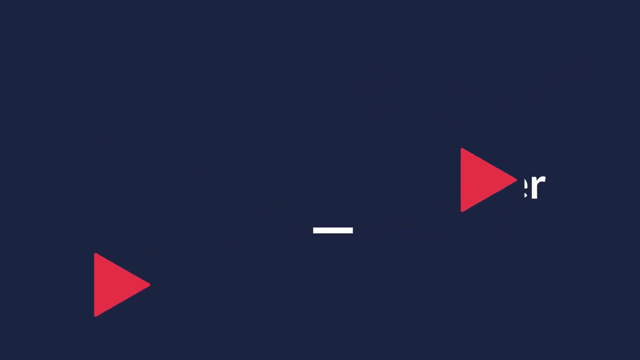 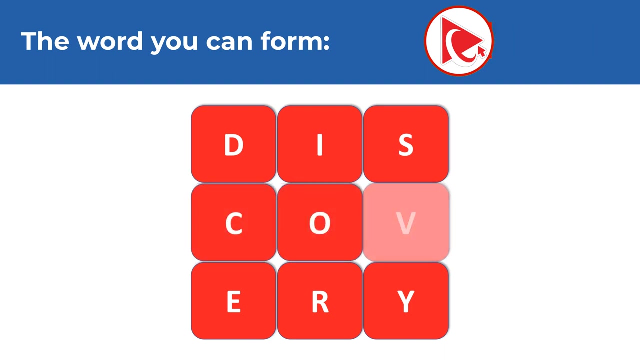 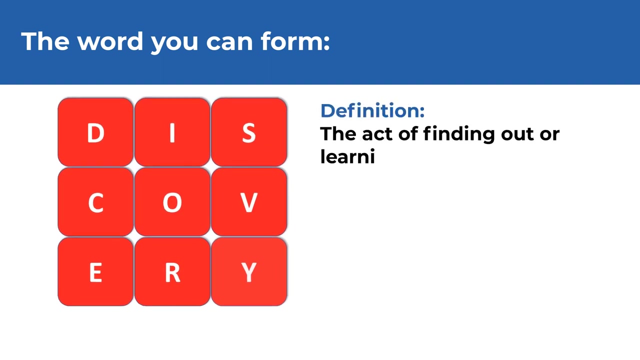 so if you see other possible options, please make sure to share them in comments. The word you can form is DISCOVERY. Let me spell it for you: D-I-S-C-O-V-I-N-G, E-R-Y, And the definition of discovery is the act of finding out or learning about something. for 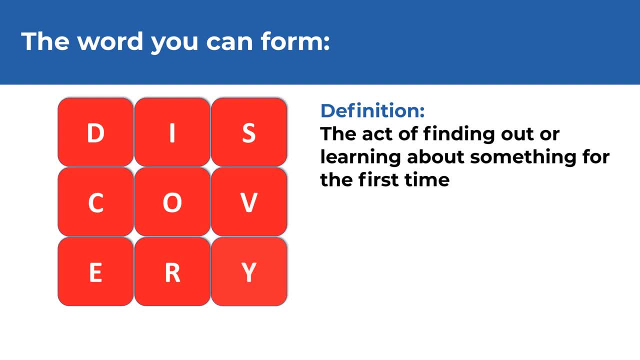 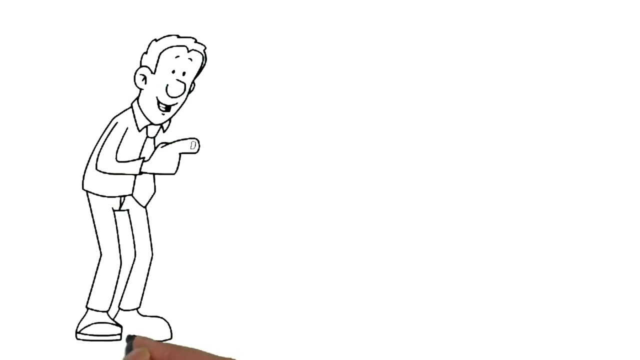 the first time. Here's the sample sentence where word discovery is used. Scientists consider detection of gravitational waves the greatest discovery of the 21st century. Did you discover any other words? Make sure to post them in comments And if you're getting ready for the 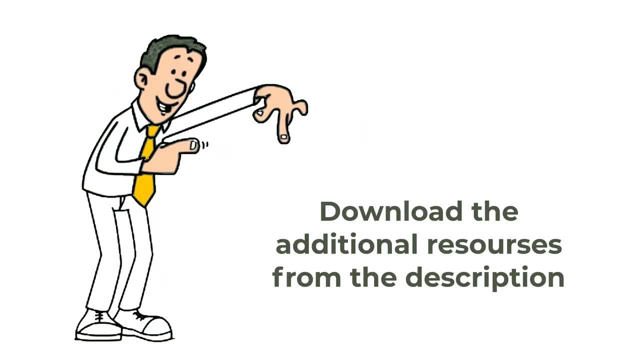 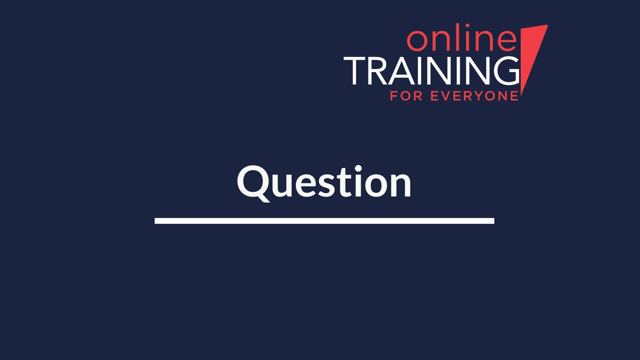 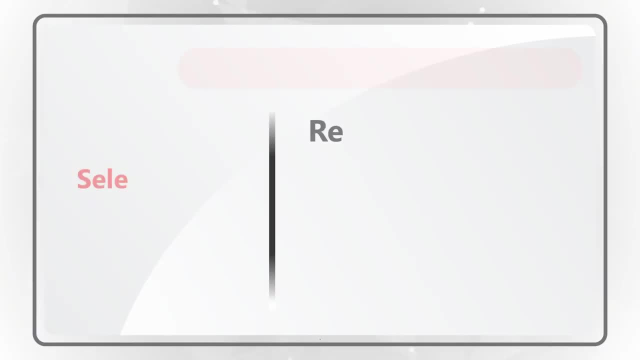 test and looking for additional questions to practice. make sure to check the description of this video For links to additional resources. Very frequently on the test, you need to identify words with the similar meaning. In this case, you're presented with five words: RECALL, VOTE, CAST, REMEMBER. 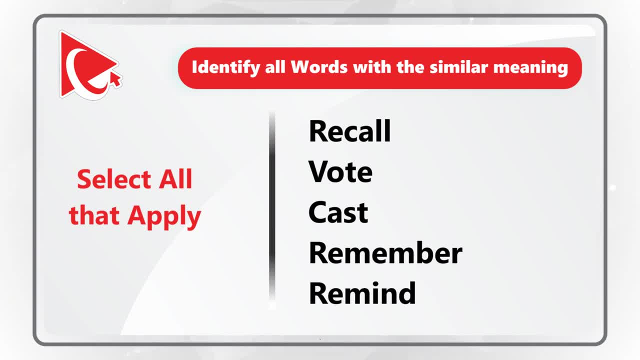 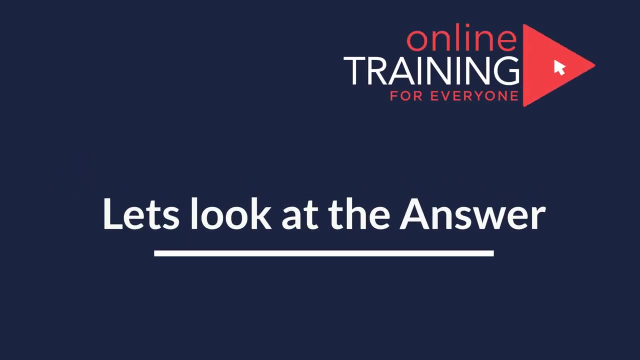 and REMIND Which words on the list have a similar meaning? Very interesting question, because the number could be between 2 and 5.. Did you get to the answer? Let's move forward and I'll show you the answer. From my standpoint, there are three words here with the similar meaning And obviously. 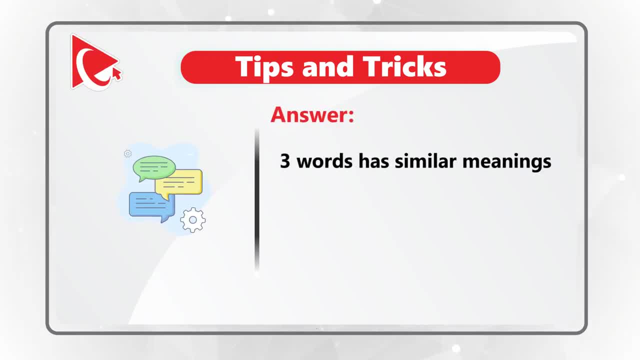 if you disagree, feel free to share your feedback in comments. But I see words RECALL, REMEMBER and REMIND having similar meaning in this particular question. To understand why we need to look at the definition. For example, word RECALL means bring something back to your mind. Word REMEMBER means 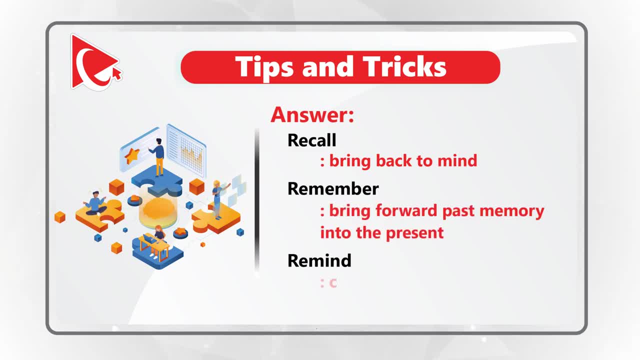 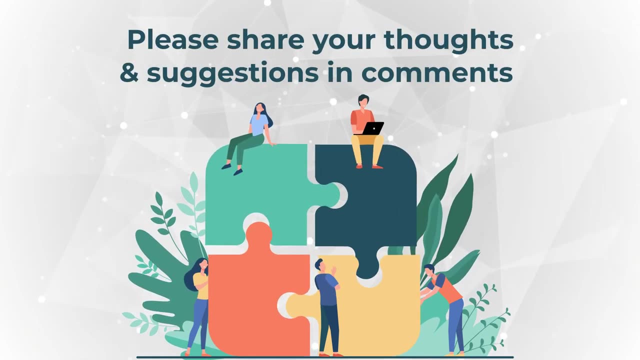 bring forward past memory into the present, And word REMIND means cause someone to remember someone or something. Not the easiest question, because each word can have multiple definitions and multiple meanings And to solve it you need to know all of them and connect them to get to. 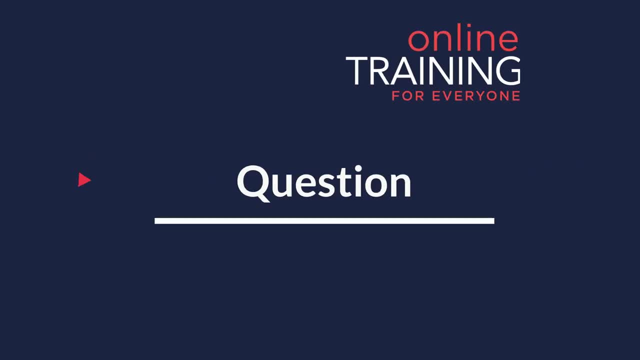 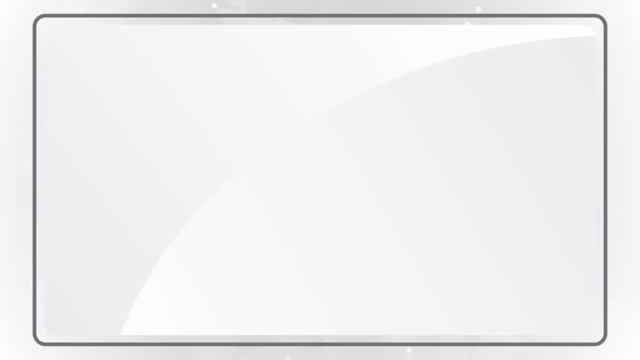 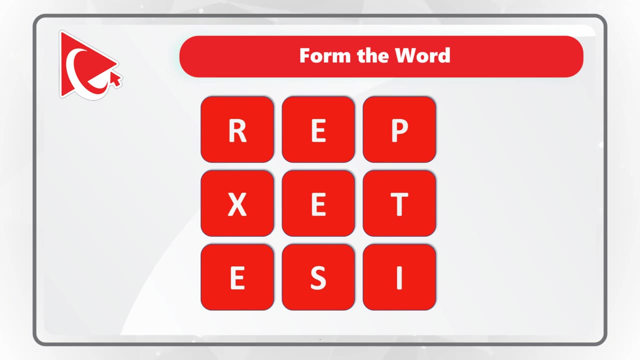 the final answer. Very frequently, you might get tested on how quickly you can form the words using letters of the English alphabet. In our case, you're presented with five words With nine letters And you need to form the word using all the letters only once The letters are. 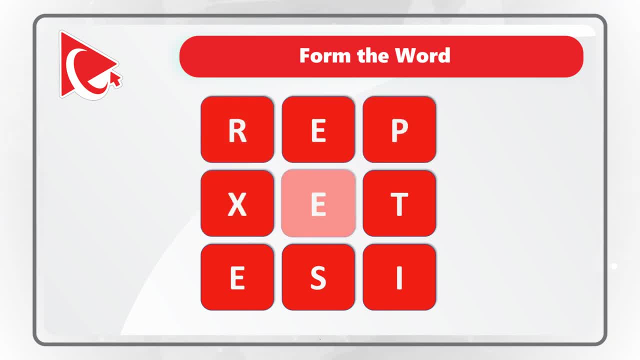 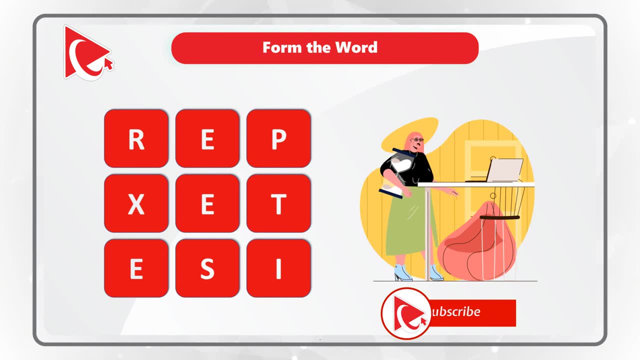 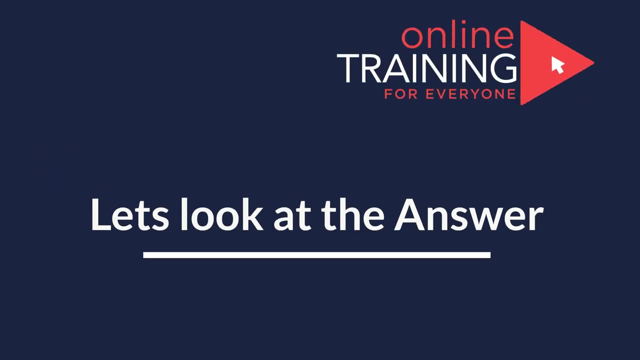 R-E-P-X-E-T-E-S-I. Do you see the word? Give yourself a little bit of time, maybe 10 to 15 seconds, to see if you can answer the question Ready or not. I am going to reveal the answer, which is the word EXPERTISE And the definition. 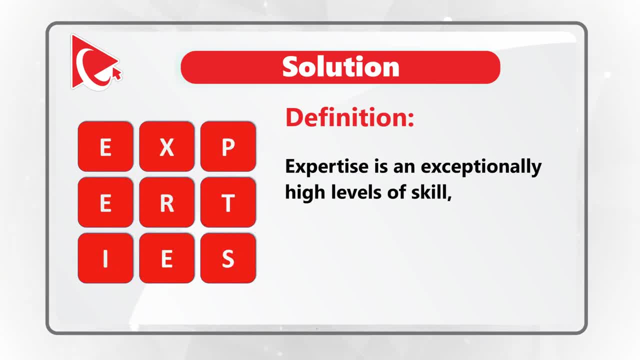 of expertise is the word EXPERTISE And the definition of expertise is the word EXPERTISE Is an exceptionally high level of skills, knowledge or performance in a particular task or within a given domain. To better solve these types of challenges, try to look at the presented 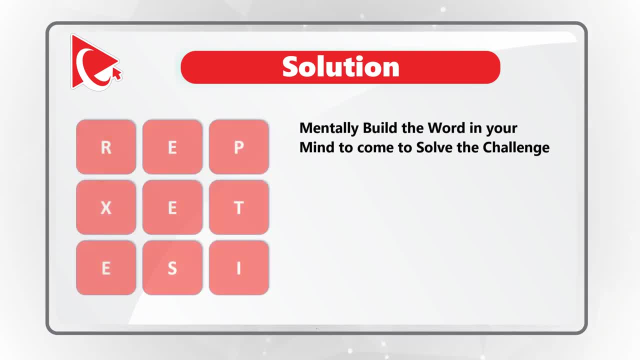 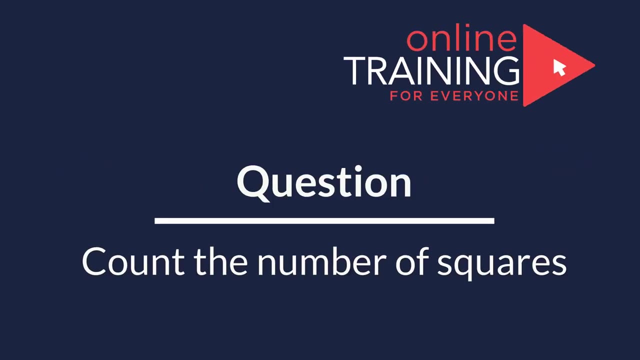 letters and try to form the word. For example, if you start in the middle and go E-X-P-E-R-T-I-S-E, you can definitely form the word EXPERTISE. Here's an interesting problem where you need to count the number of squares. 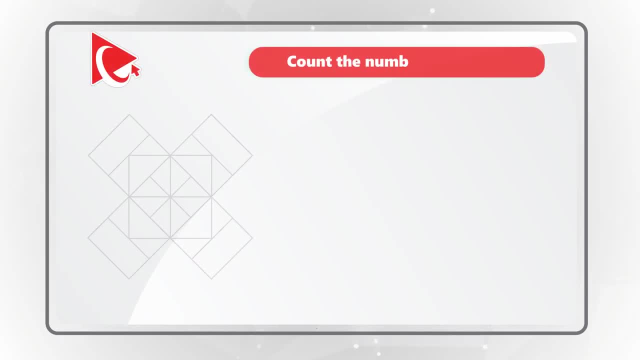 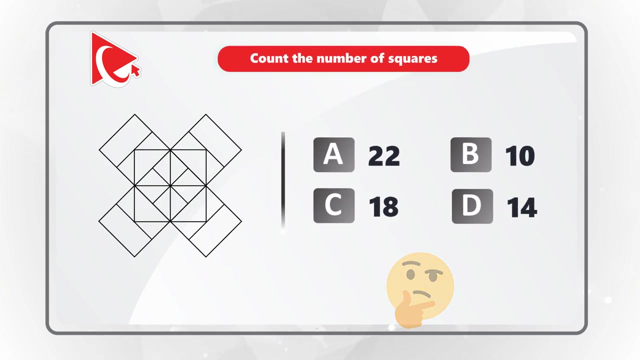 In the presented shape, the correct number is one of four different choices: Choice A: 22.. Choice B: 10.. Choice C: 18. And choice D: 14.. Take a close look at the picture to see if you can come up with the right solution. 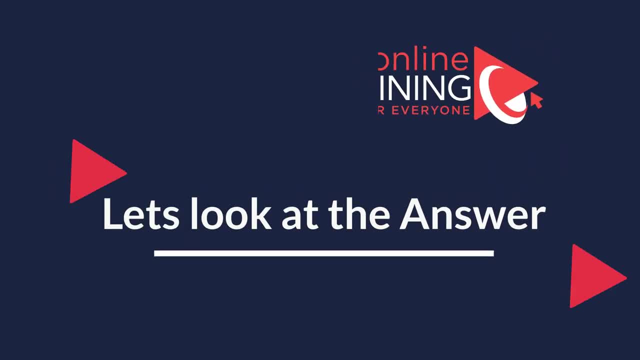 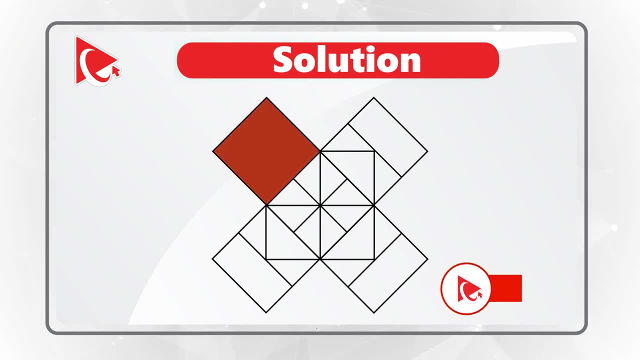 I was really impressed, but there are 18 squares in this picture. Let me show them all to you. Watch carefully and try to understand what you have to think. One, two, three, four, five, six, seven, eight, nine, ten, eleven, twelve, thirteen, fourteen. 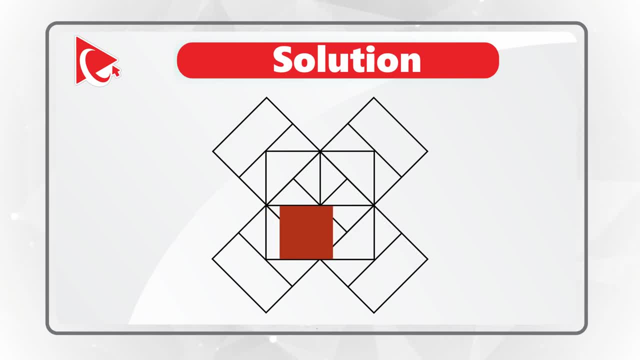 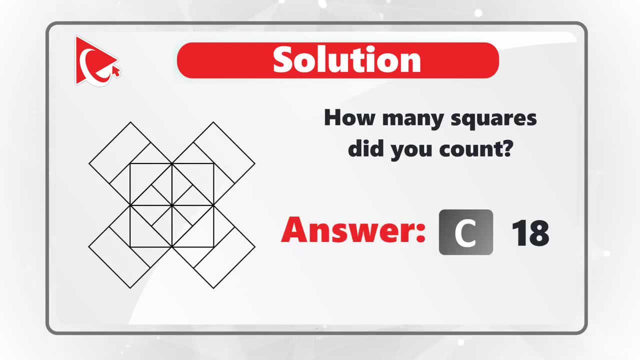 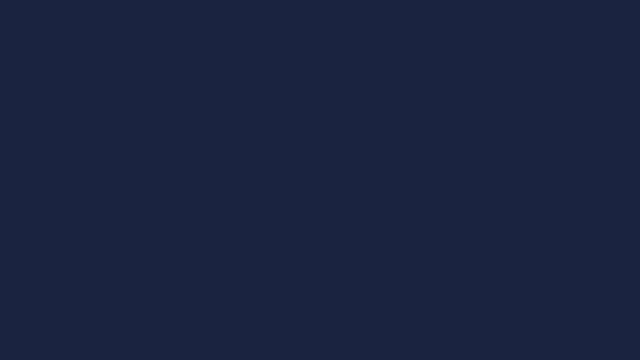 fifteen, sixteen, seventeen and eighteen. Do you see any additional ones? It is totally possible that I missed one of the squares, And if you do see any additional ones, please make sure to post them in comments. And now here is the question for you to try your skills. 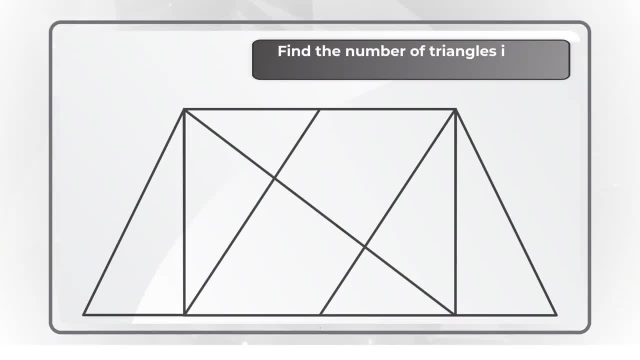 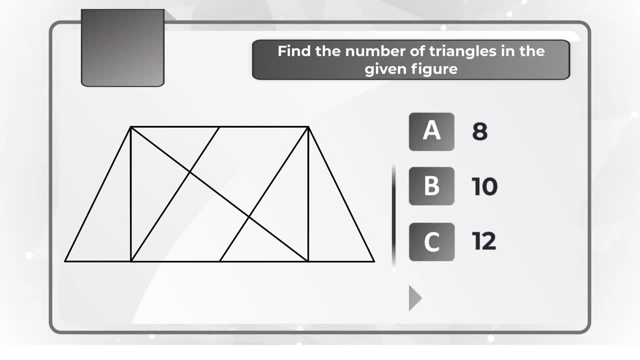 You need to determine how many triangles are shown on the screen. You have four different choices: Choice A – 8,, choice B – 10,, choice C – 12, and choice D – 14.. Feel free to pause this video to calculate the right answer. 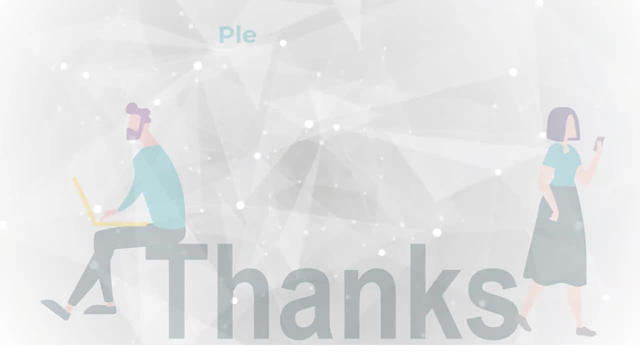 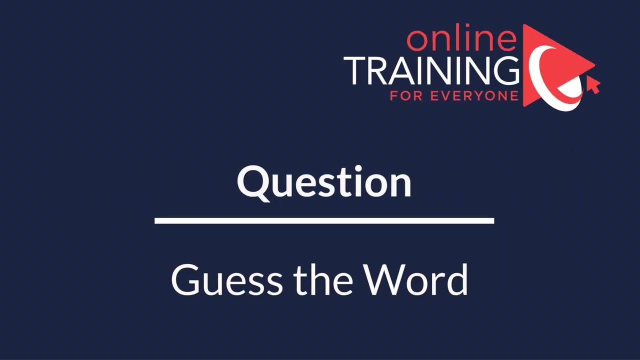 And make sure to post your solution in comments so I can give you my feedback. Thanks for participating and good luck. Here is an interesting question from the recent test. You need to figure out the word from the five letters you see on the screen. 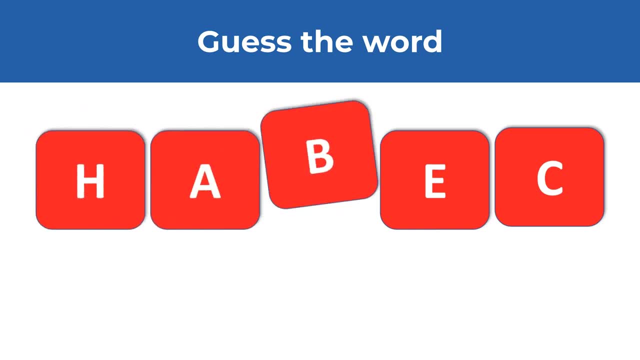 The letters are H, A, B, E and C. Do you see the word? Give yourself 10 to 15 seconds, maybe 20 seconds. You can pause this video to see if you can figure it out on your own. 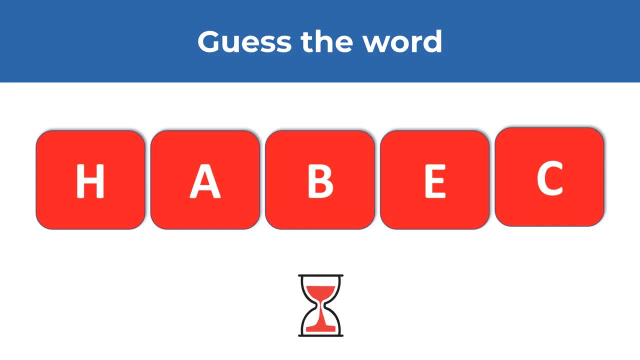 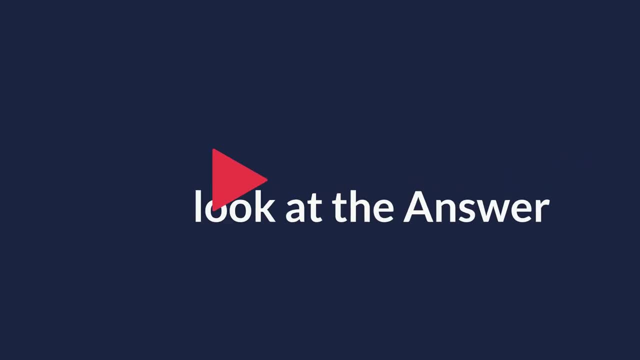 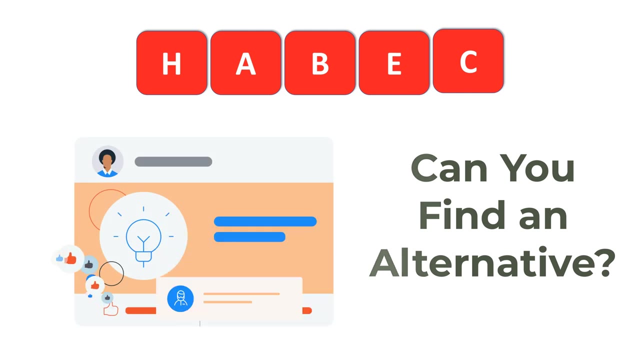 Make sure to use all the letters and make sure to use each of the letters once Ready or not. I am going to move forward and share with you my solution, But keep in mind that a lot of times, multiple words can be formed, So if you see another word, please make sure to share it in comments. 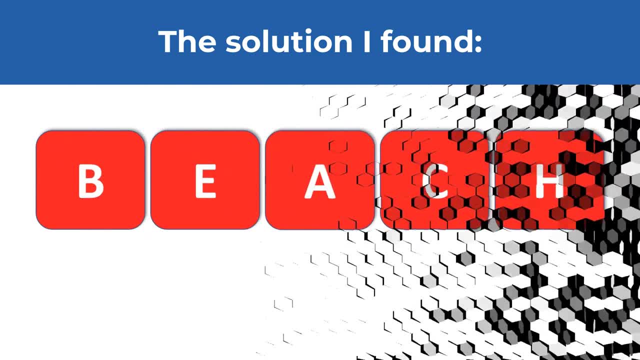 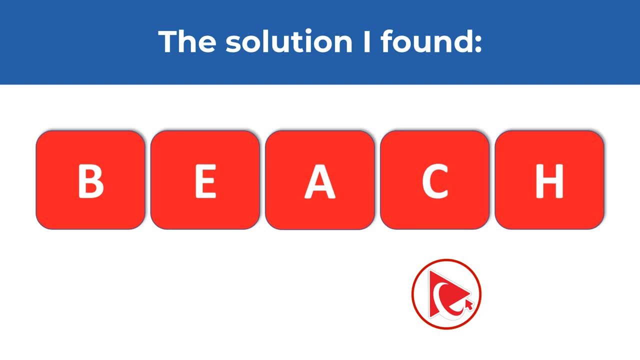 The solution I found is the word beach. Let me spell it for you – B-E-A-C-H. Do you see any other solutions? Make sure to post them in comments, And if you'd like to improve your ability to guess the words, you can play word games. 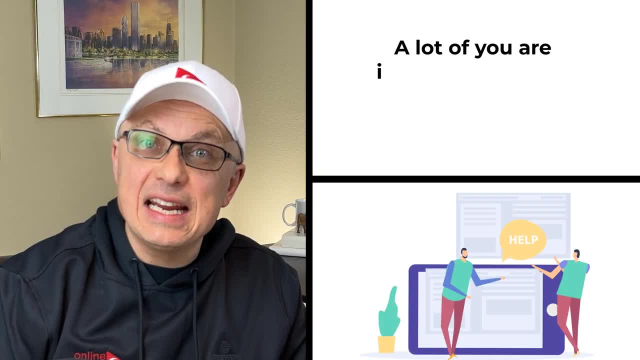 read a lot and practice crosswords and puzzles. A lot of you are interested and ask me: how can I help others? One of the ways you can help other people is by following the link in the description of this video, And if you have any questions, please share them in the comments section of this video. 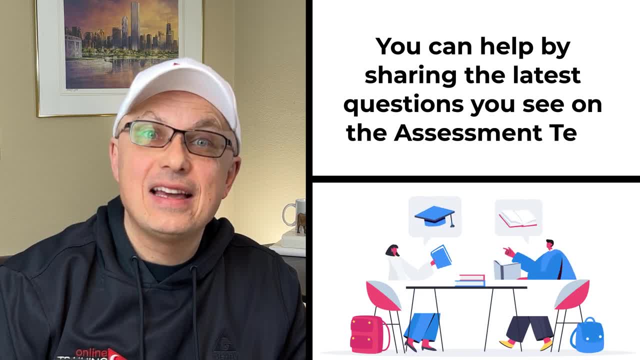 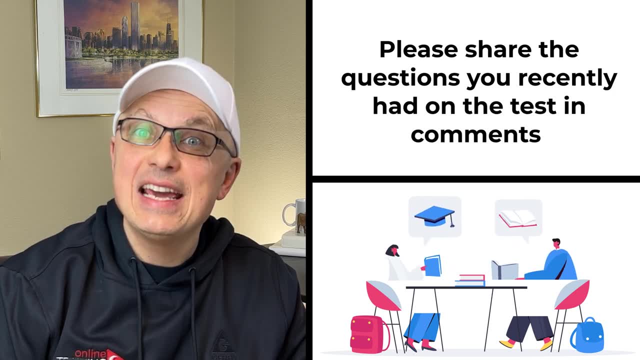 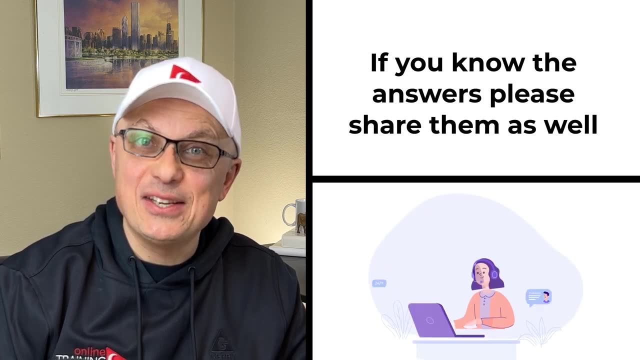 And when you share, please make sure to also include how you answered them. Please share the question you recently encountered in the comments section of this video And if you know the answers, please share them as well. And now let's continue and get you ready for the test. 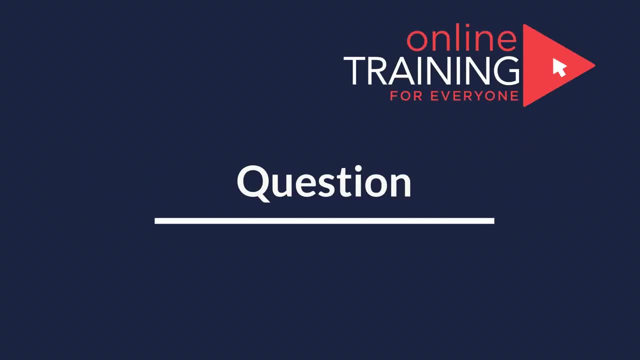 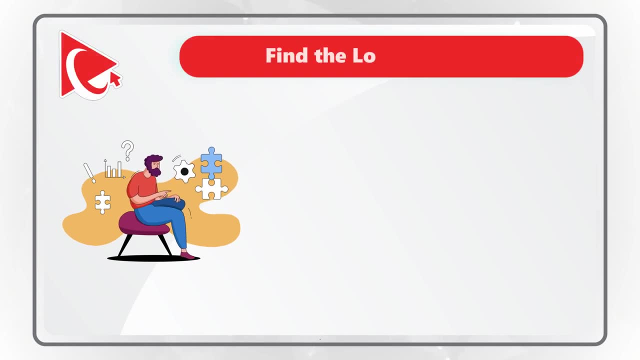 I love this question because it truly makes you think. to determine the final answer, You need to determine which number has the lowest value, And you have four different choices. Choice A: 1 third plus 0.4.. Choice B: 1 plus 2.1.. 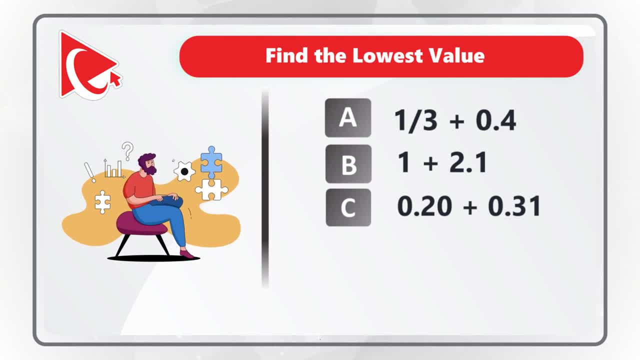 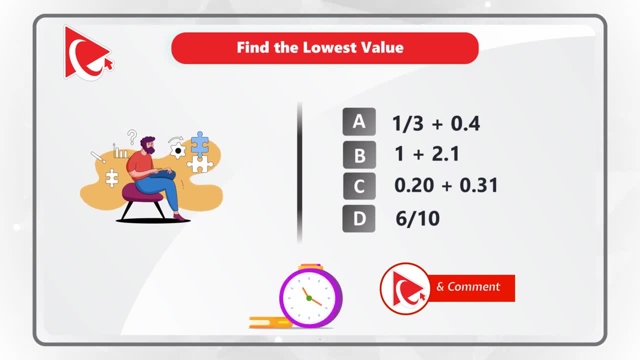 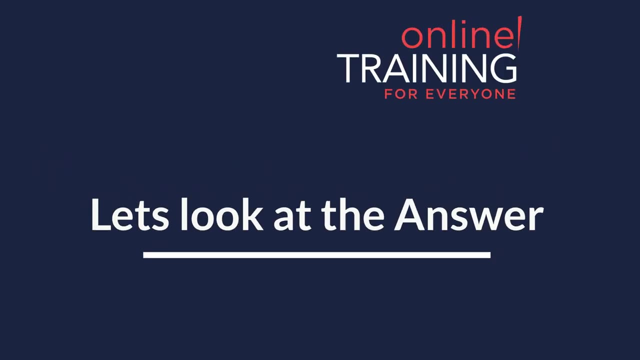 Choice C: 0.2 plus 0.31.. And choice D: 6 tenths. Give yourself a few seconds to see if you can come up with the solution. The tricky part here is that the question is designed to make you do a mental math. 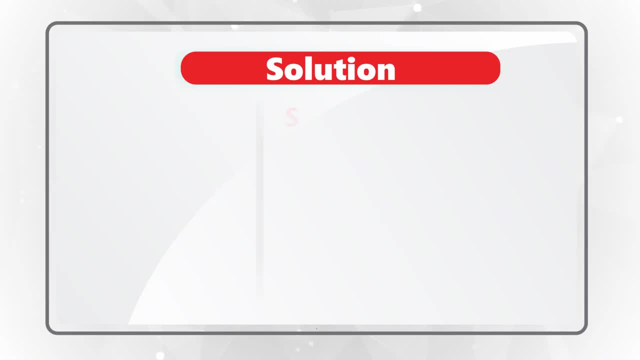 To get to the final answer, You need to simplify all the options. For example, option A: 1, third plus 0.4, equals 0.33 plus 0.4, which is 0.73.. Choice B: 1 plus 2.1 equals 3.1.. 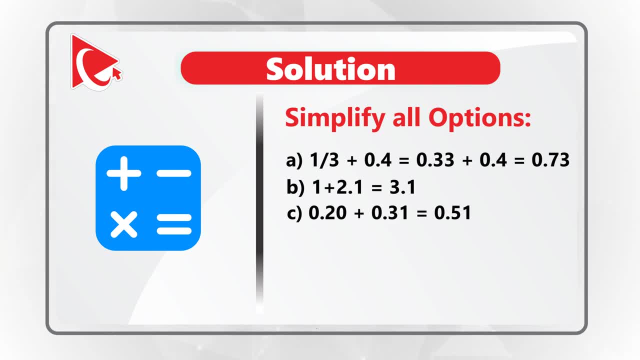 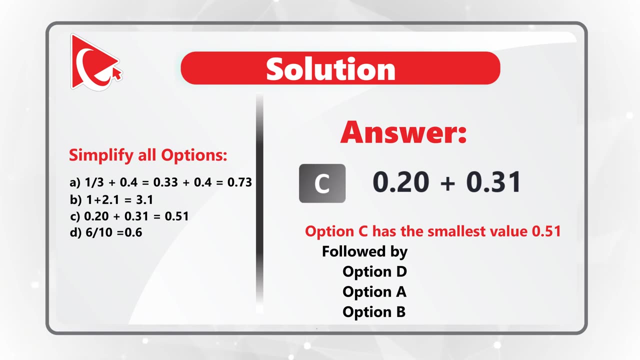 Choice C: 0.20 plus 0.31 equals 0.51.. And choice D: 6 tenths equals 0.6.. Which means That option C has the smallest value of 0.51.. Followed by option D, A and B. 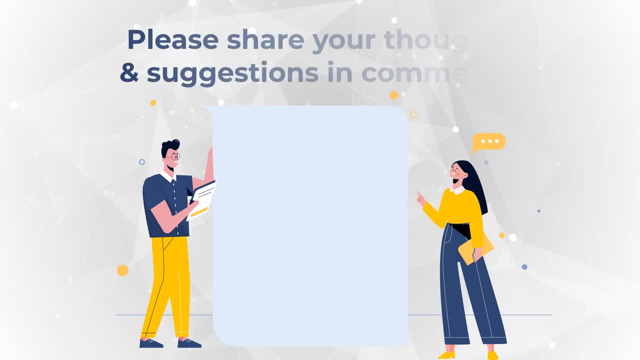 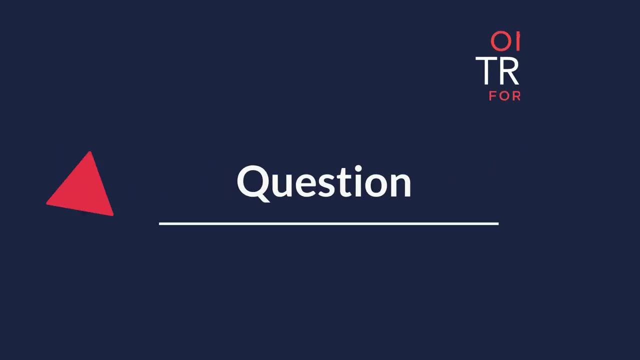 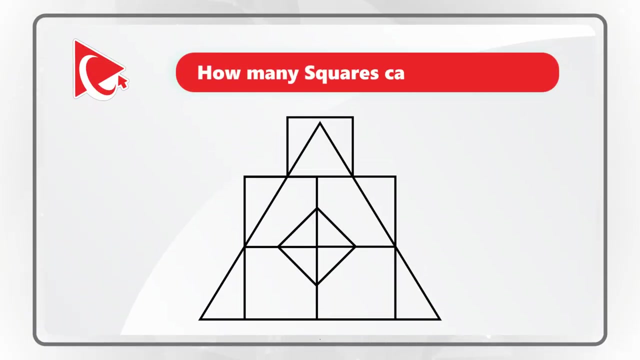 Was it challenging for you. Please share your thoughts and suggestions on how to better solve it in comments. Here is an interesting question where you need to correctly count the number of squares on a picture. Take a close look and select from one of the following choices: 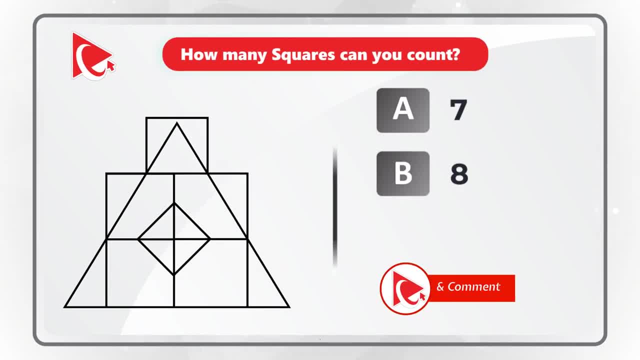 Choice A: 7 squares, Choice B: 1 third plus 0.51.. Choice B: 8 squares, Choice C: 9 squares And choice C: 12 squares. Make sure to count inside and outside squares to get to the correct solution. 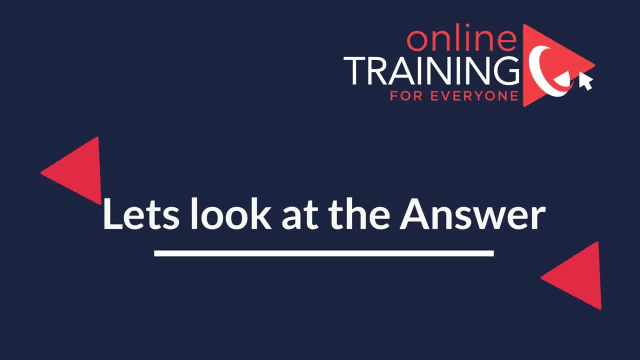 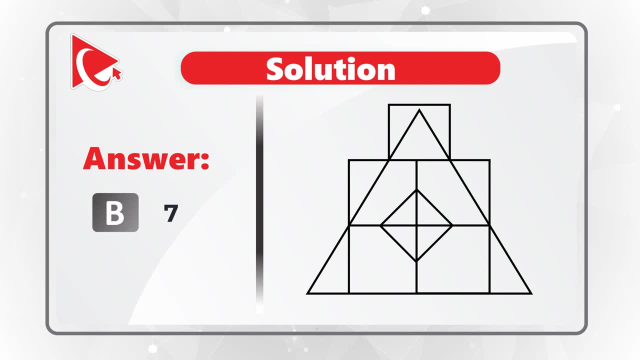 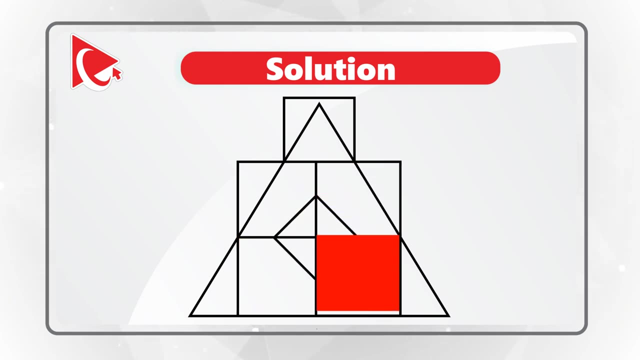 Let me show you the final answer. I counted 7 squares on a picture. Obviously, if you have a different answer, please make sure to post your solution in comments. Here are all the squares: 1., 2., 3., 4.. 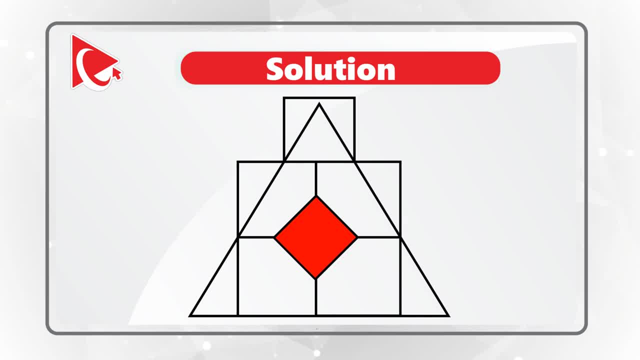 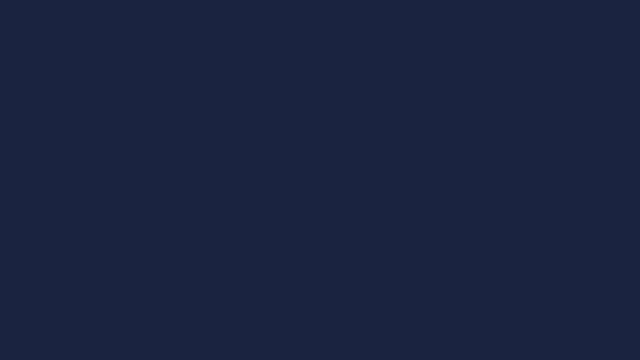 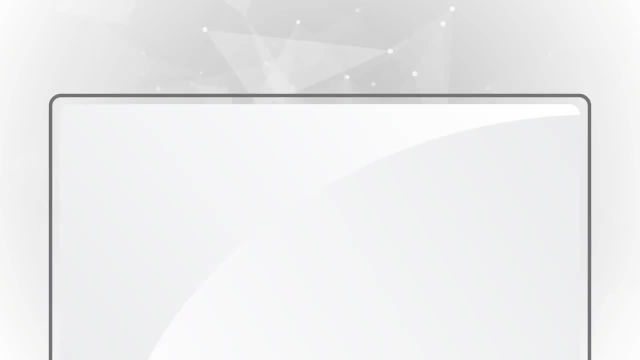 5., 6. And 7.. Do you have a different number? I am looking forward to your response. if you counted more or less squares, Here is the interesting challenge you might frequently see on the test. You need to determine minimum time for people to cross the bridge. 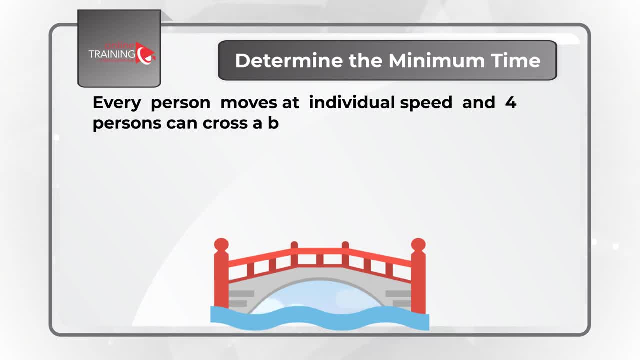 Every person moves at individual speed and 4 people can cross the bridge in different durations. They can cross it in 3,, 7,, 13 and 17 minutes respectively. The trick here is that only two people can cross the bridge at the same time. 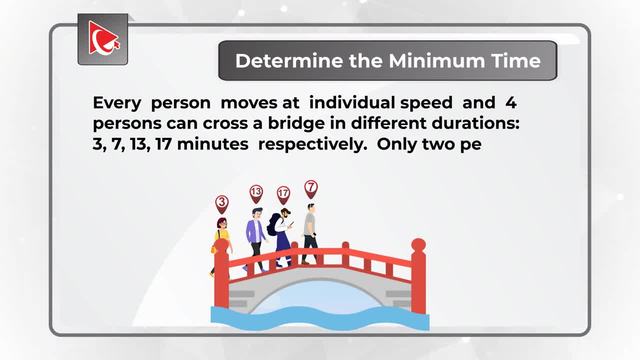 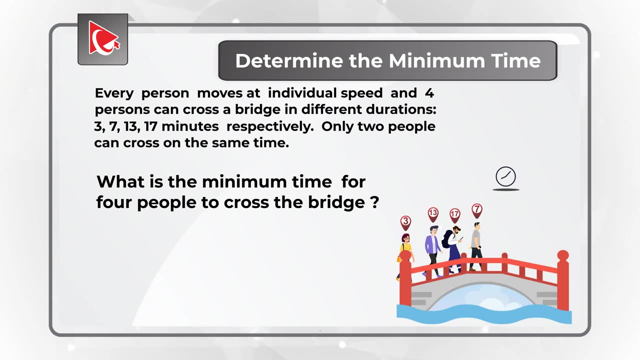 In this example, only 2 person의 people can cross the bridge at the same time. You need to determine what is the minimum time for 4 people to cross the bridge. You are presented with 4 different choices. Choice A: 17 minutes. 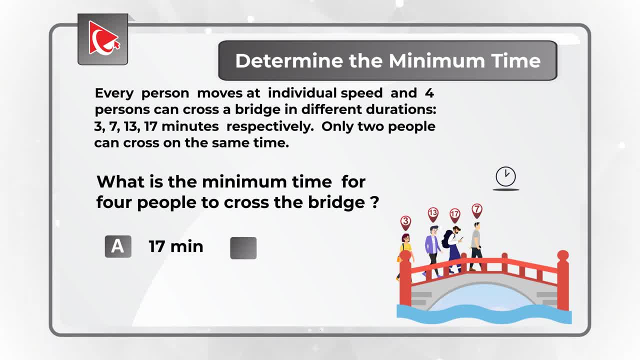 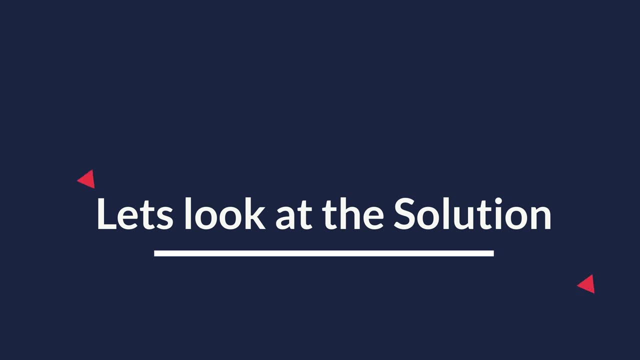 Choice B: 20 minutes. Choice C: 30 minutes. 2. 3. 34 minutes and choice D: 12 minutes. Are you ready for the challenge? Let's move forward and get to the correct solution together, As you might have determined certain sequence. 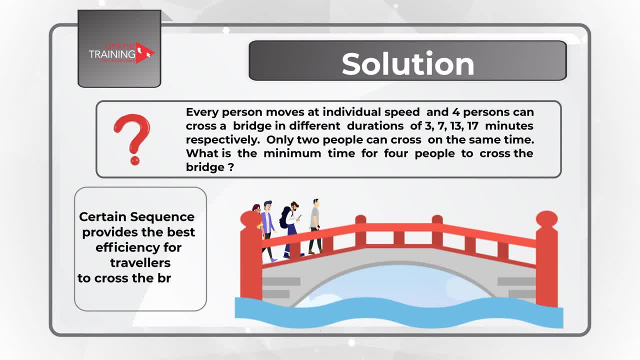 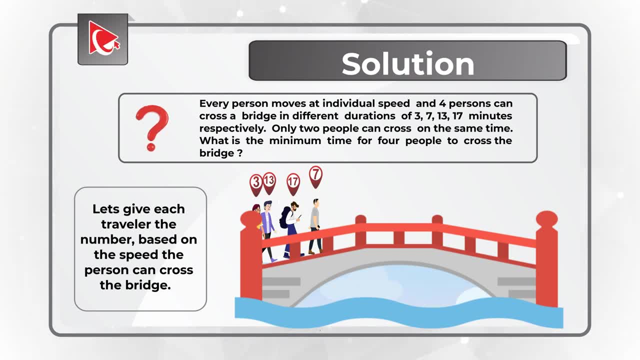 provides the best efficiency for travelers to cross the bridge. Let's give each traveler the number Based on the speed this person can cross the bridge. We will first send number 17 and 7 at the same time to cross the bridge. After 7 minutes, number 7 finished crossing the bridge. 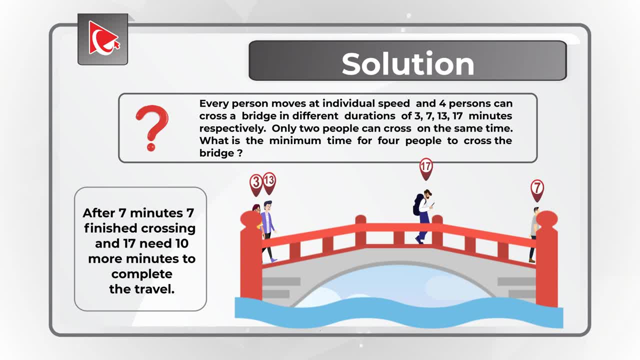 and number 17 needs additional 10 minutes to complete the travel. Let's now send number 13.. After additional 10 minutes, number 17 reaches the finish line and number 13 needs 3 more minutes to complete the travel. Let's now send number 3.. 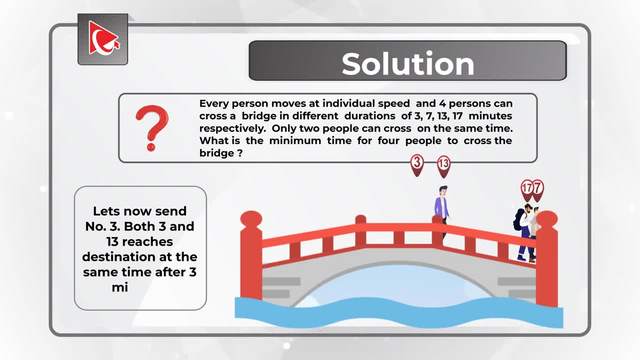 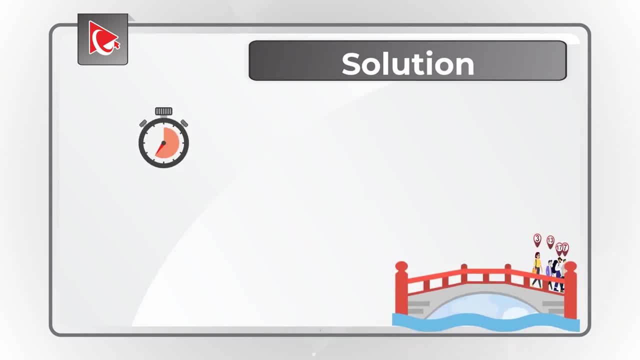 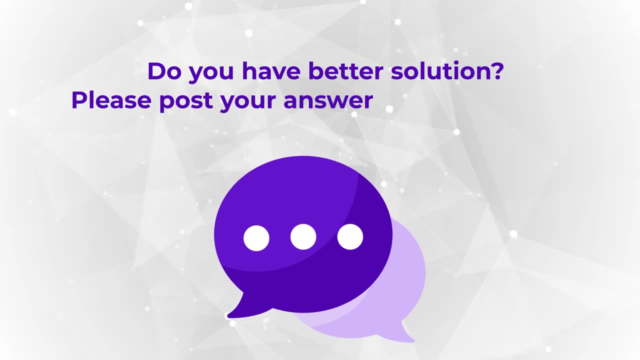 Both number 3 and number 13 reach destination at the same time after additional 3 minutes, And total time it took for travelers to cross the bridge would be 7 plus 10 plus 3 equals 20 minutes. So the correct answer here is choice B, 20 minutes. Hopefully you've nailed this question and now know. 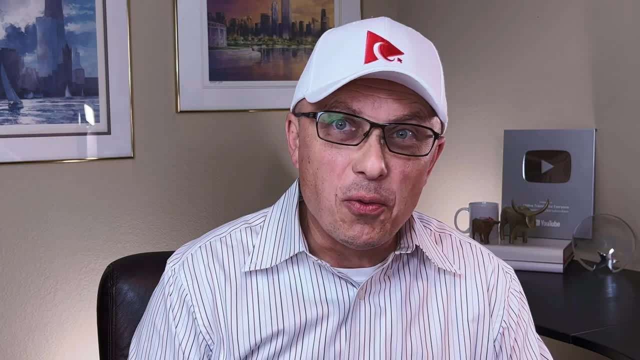 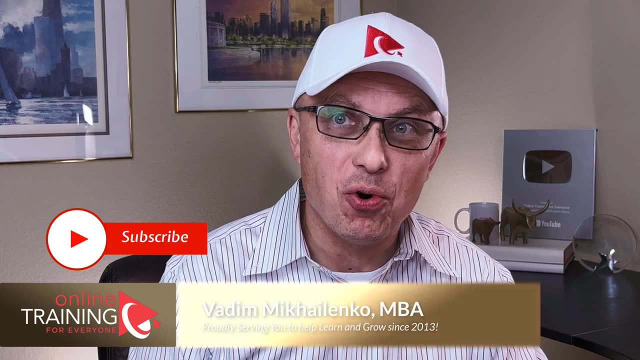 how to answer similar problems on the test. Thanks for watching. If you liked the content, please give us a like and consider subscribing. Thanks for all your endorsement, support and patronage. For additional helpful information, please make sure to check out links in the. 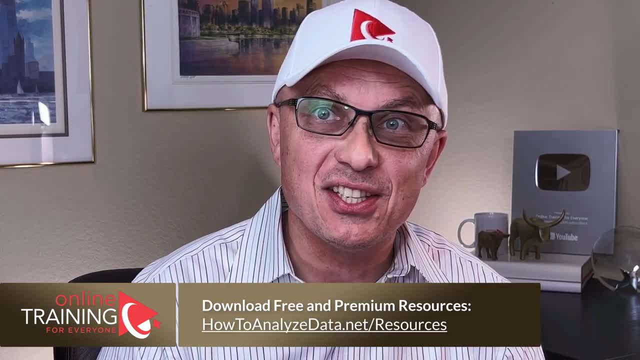 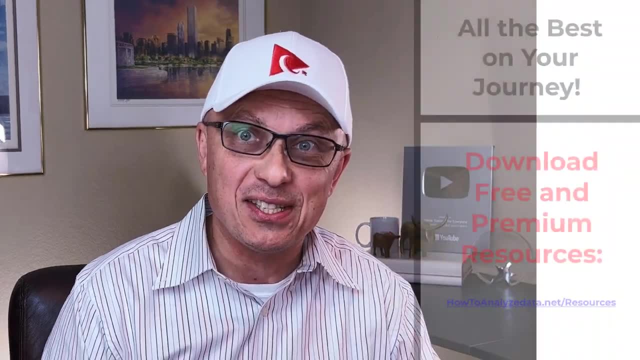 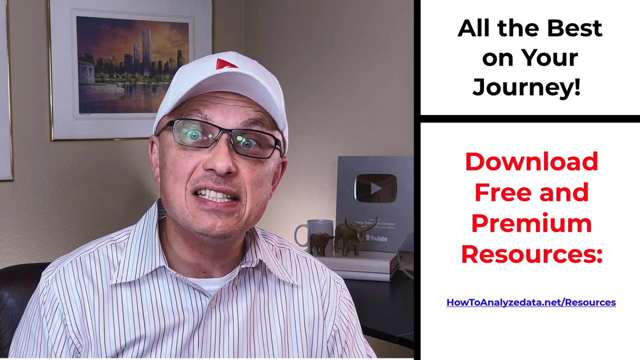 description For detailed list of available resources. I encourage you to check out resources page on our website, howtoanalyzedatanet slash resources. If you know someone who would benefit from this content, please consider sharing the link. Please leave the feedback correctly. 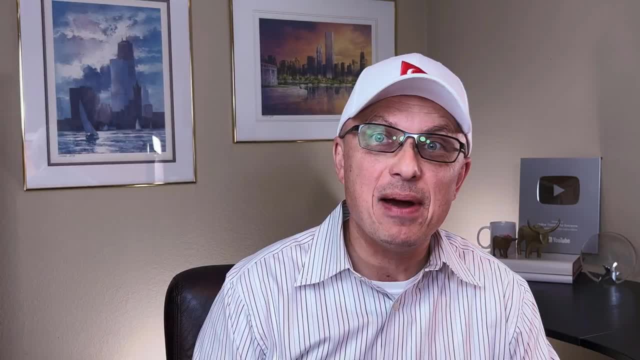 suggestions or suggestions in comments, And all the best on your journey. I'll see you in my next video.